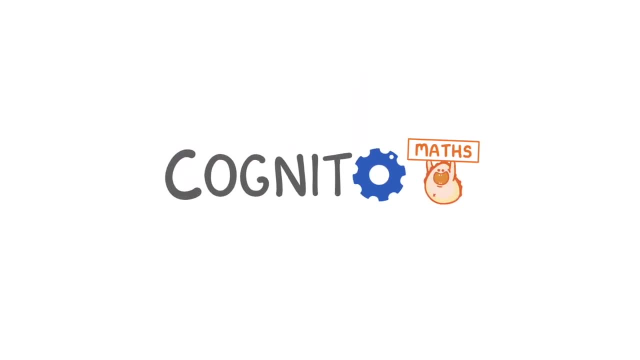 In this video we're going to cover how to solve basic algebraic equations where there's only one unknown letter. We can see this if we look at these two equations: In this left one, the only unknown letter is this x, and in this right one, the only unknown letter is the a. When you're asked, 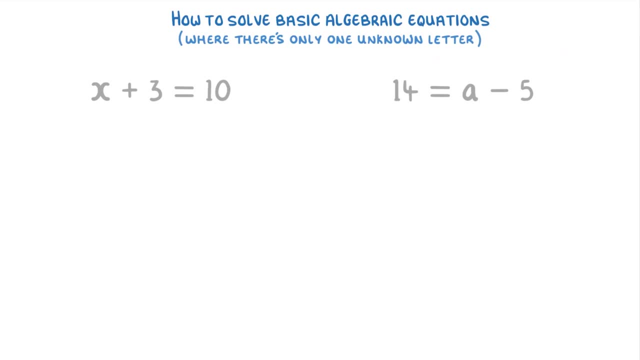 to solve equations like these, you're really being asked to find out what number the unknown letter represents. So in this first one, we're being told that something plus 3 equals 10, and we have to find out what that something is. Now you might just know automatically that the 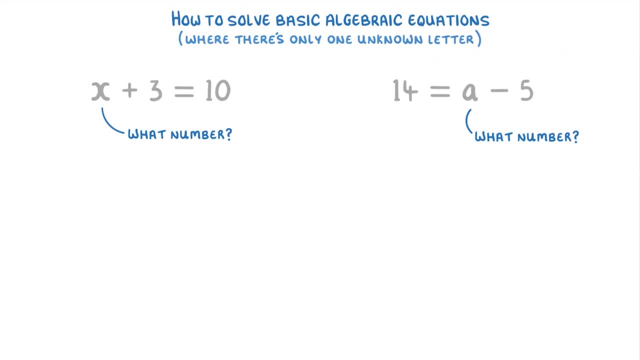 answer here is 7,, because you know that 7 plus 3 equals 10.. Most of the time, though, the questions will be a bit trickier, and in order to find the answer, you'll have to rearrange the equation to get that unknown letter all by itself. Whenever you rearrange equations, though, 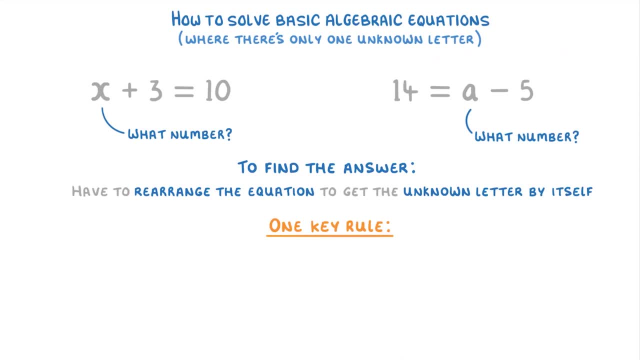 there's one key rule that you have to remember, which is that whatever you do to one side of the equation, you have to do to the other side of the equation as well. If you don't do this, then the two sides won't actually be equal to each other anymore. 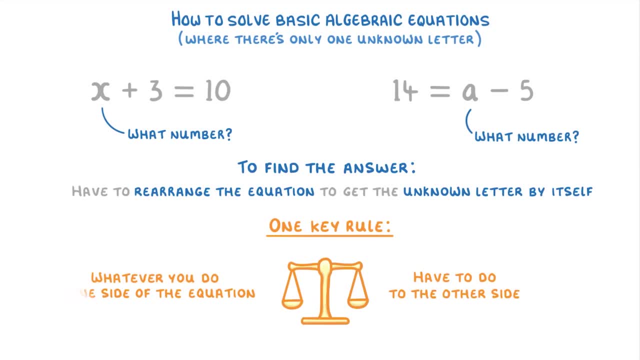 and the equation won't be correct. So for this first equation, in order to get the x by itself, we need to get rid of this 3.. At the moment, the 3 is being added to our x, So if we want to get rid of it, 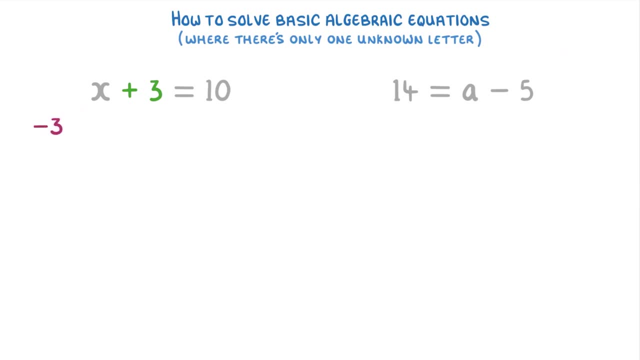 we're going to have to do the opposite and subtract 3.. However, if we subtract 3 from the left-hand side, then we're also going to have to subtract 3 from the right-hand side, because we're going to have to subtract 3 from the left-hand side. 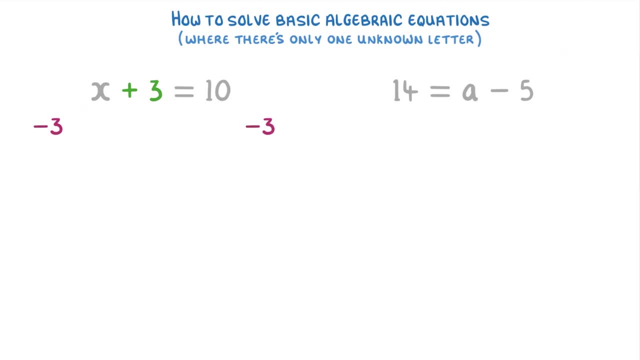 Because, remember, we always have to do the same thing to both sides. It's completely up to you how you want to show this, but one of the most common ways, and the way that I think is probably easiest, is to put a little arrow on either side of the 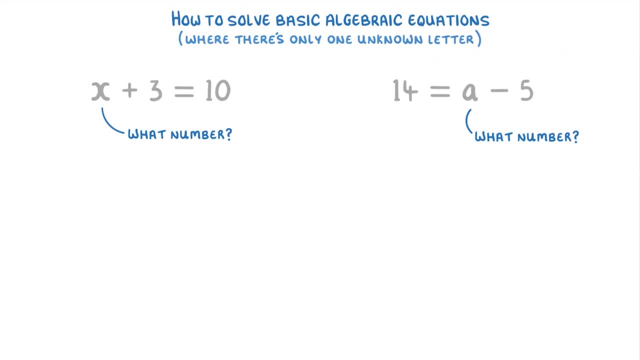 answer here is 7,, because you know that 7 plus 3 equals 10.. Most of the time, though, the questions will be a bit trickier, and in order to find the answer, you'll have to rearrange the equation to get that unknown letter all by itself. Whenever you rearrange equations, though, 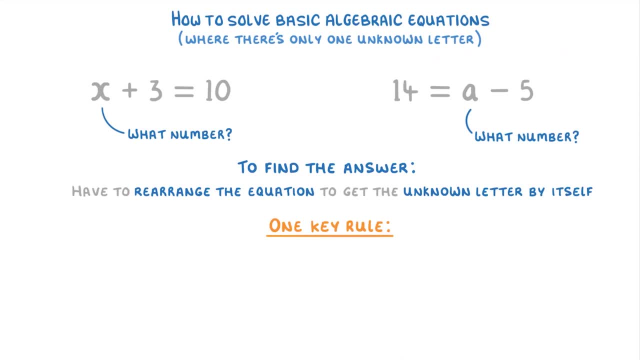 there's one key rule that you have to remember, which is that whatever you do to one side of the equation, you have to do to the other side of the equation as well. If you don't do this, then the two sides won't actually be equal to each other anymore. 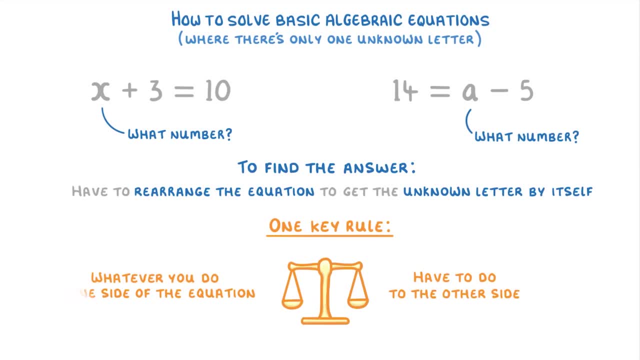 and the equation won't be correct. So for this first equation, in order to get the x by itself, we need to get rid of this 3.. At the moment, the 3 is being added to our x, So if we want to get rid of it, 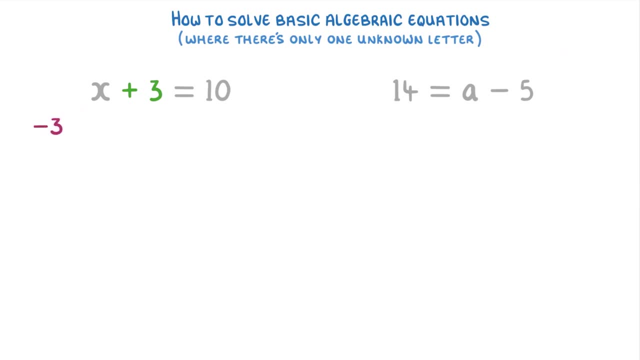 we're going to have to do the opposite and subtract 3.. However, if we subtract 3 from the left-hand side, then we're also going to have to subtract 3 from the right-hand side, because we're going to have to subtract 3 from the left-hand side. 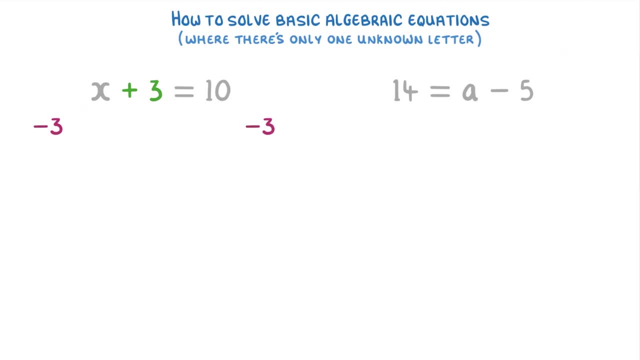 Because, remember, we always have to do the same thing to both sides. It's completely up to you how you want to show this, but one of the most common ways, and the way that I think is probably easiest, is to put a little arrow on either side of the 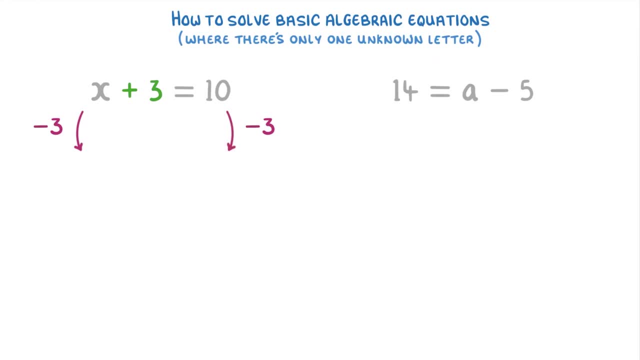 equation and put a minus 3 next to them both so that you know to subtract 3 from both sides. You won't get any marks for this in the exam, but it helps for more complicated questions where it's really easy to get confused. 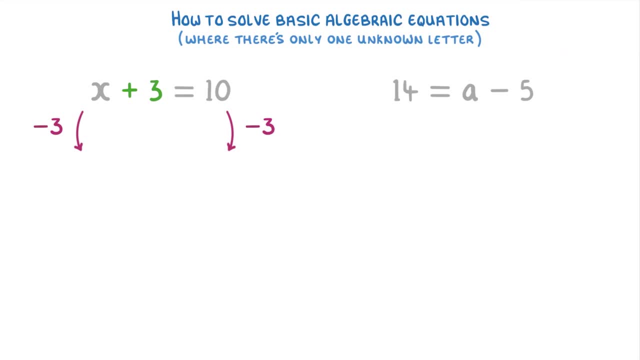 So if we subtract this 3 from the left side, then it'll get rid of the 3 that we already have and we'll be left with just x on the left. Then, for the right, 10 minus 3 is 7, so we just put 7.. 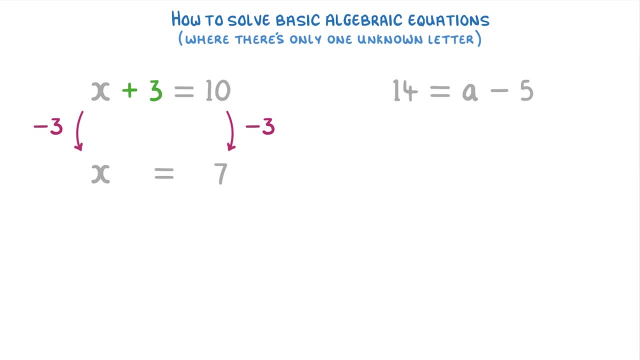 And we now have our answer that x equals 7.. Let's have a go at this second one, where 14 is equal to a minus 5.. To get the a by itself, we need to get rid of this minus 5 term. 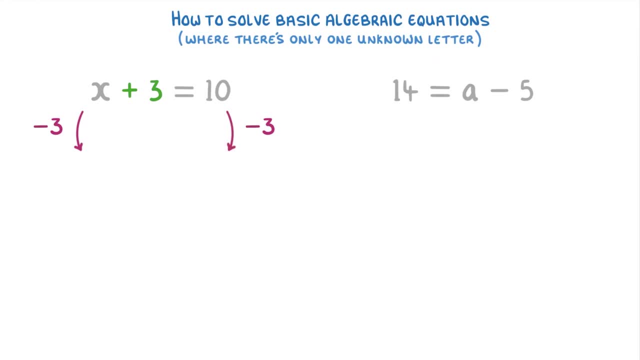 equation and put a minus 3 next to them both so that you know to subtract 3 from both sides. You won't get any marks for this in the exam, but it helps for more complicated questions where it's really easy to get confused. 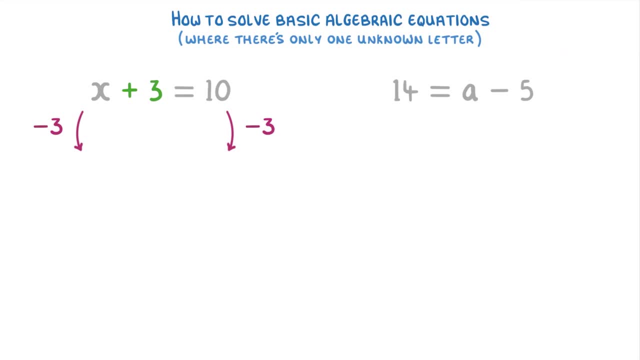 So if we subtract this 3 from the left side, then it'll get rid of the 3 that we already have and we'll be left with just x on the left. Then, for the right, 10 minus 3 is 7, so we just put 7.. 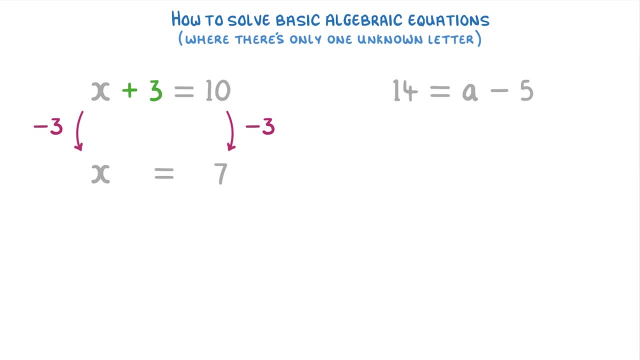 And we now have our answer that x equals 7.. Let's have a go at this second one, where 14 is equal to a minus 5.. To get the a by itself, we need to get rid of this minus 5 term. 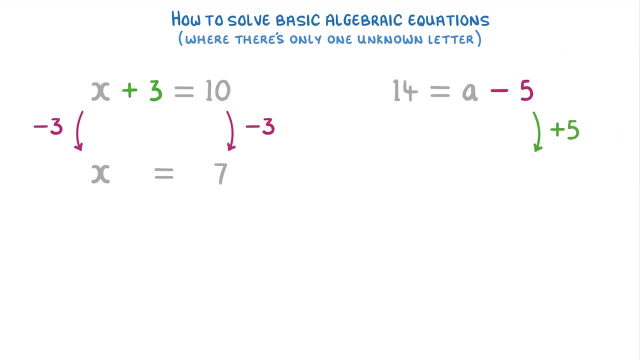 So we're going to have to do the opposite and add 5.. But remember, we have to add 5 to both sides. On the left, this gives us 14 plus 5, which is 19. And on the right, the minus 5 and the plus 5 cancel each other out. so we're left with just a. 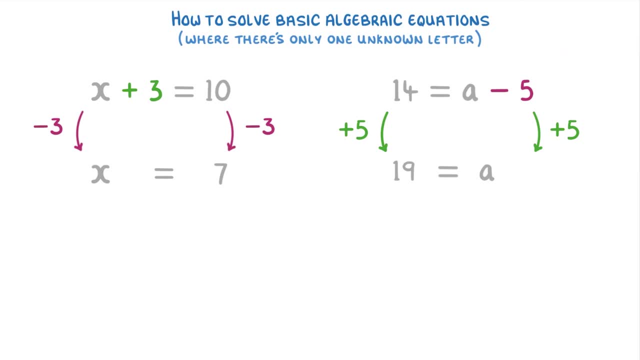 Which means that a must equal 5. Or 19.. Next, we need to look at equations that involve multiplication and division. The idea for these is exactly the same: We want to get the unknown letter by itself, and whatever we do to one side, we have to do to the other. 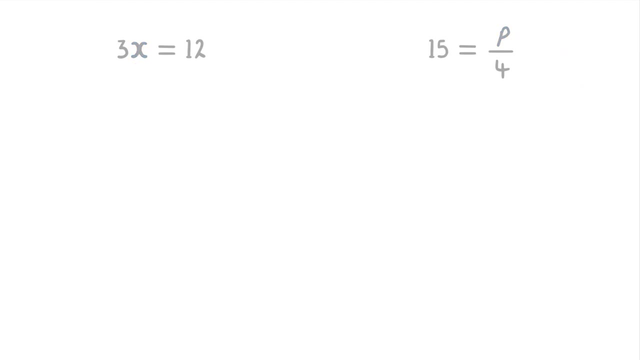 So in this first one, to get x by itself, we need to get rid of this 3.. As the x is currently being multiplied by it, to get rid of it we're going to have to do the opposite and divide by 3. So we need to divide. 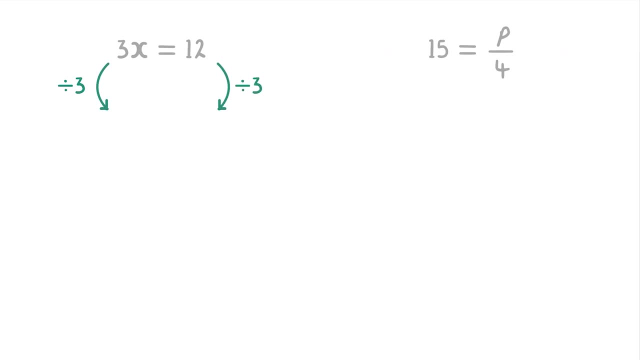 both sides by 3.. On the left, 3x divided by 3 gives us 1x or just x, and then on the right we do 12 divided by 3 to get 4.. So x must equal 4.. For this next one, we're told that 15 is equal to. 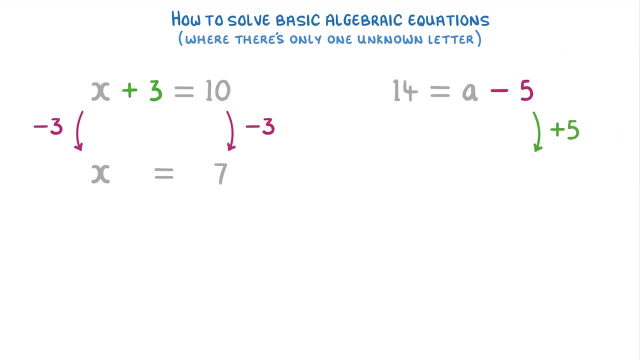 So we're going to have to do the opposite and add 5.. But remember, we have to add 5 to both sides. On the left, this gives us 14 plus 5, which is 19. And on the right, the minus 5 and the plus 5 cancel each other out. so we're left with just a. 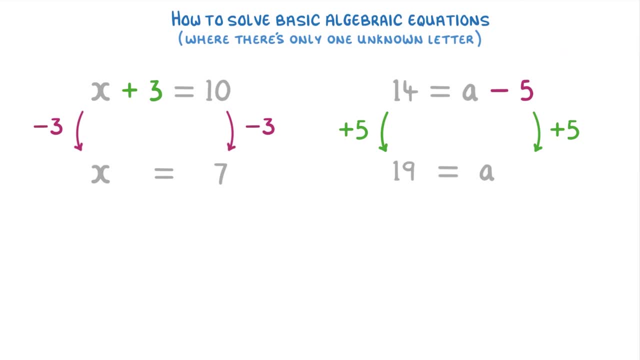 Which means that a must equal 5. Or 19.. Next, we need to look at equations that involve multiplication and division. The idea for these is exactly the same: We want to get the unknown letter by itself, And whatever we do to one side, we have to do to the other. 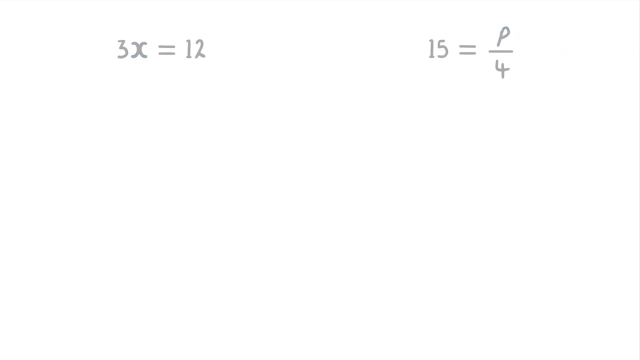 So in this first one, to get x by itself, we need to get rid of this 3.. As the x is currently being multiplied by it, to get rid of it we're going to have to do the opposite and divide by 3.. 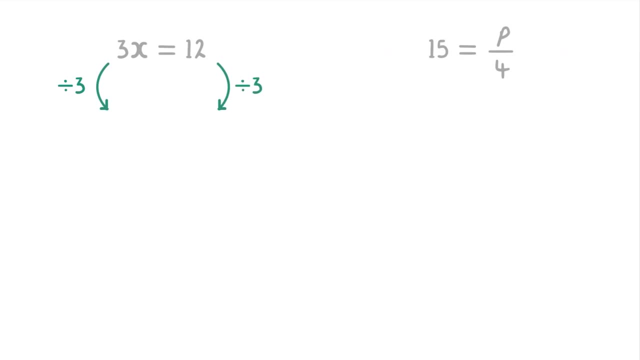 So we need to divide both sides by 3.. On the left, 3x divided by 3 gives us 1x or just x, And then on the right we do 12 divided by 3 to get 4.. 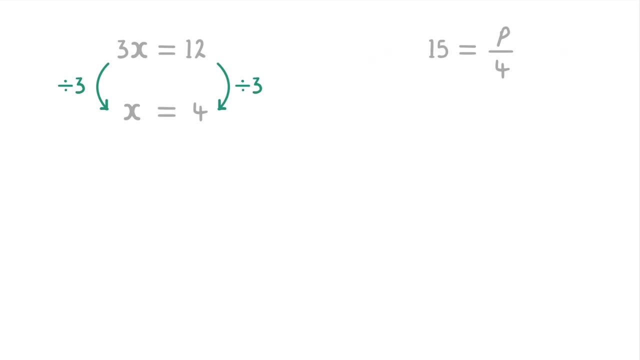 So x must equal 4.. For this next one, we're told that 15 is equal to p divided by 4. So to get the p by itself, we're going to have to do the opposite and multiply both sides by 4.. 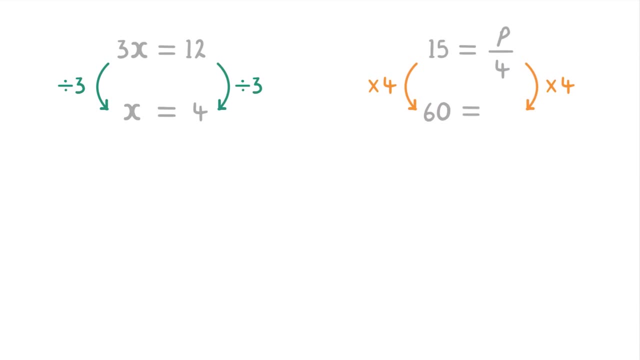 15 times 4 is 60. And on the right, the divide by 4 and the multiply by 4 will cancel out. So we're left with 60 equals p. Let's try two more quick ones. This first one. 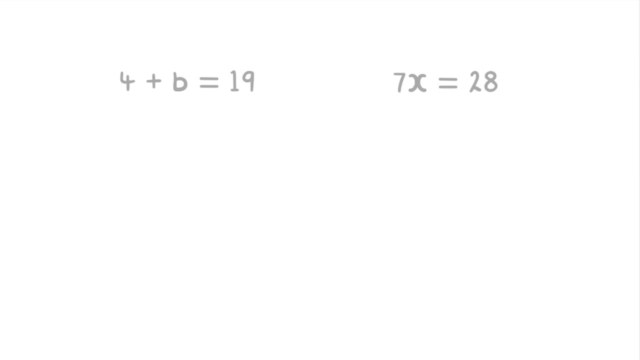 4 plus b equals 19, is a bit different to the other ones we've seen so far, Because there's no sign in front of the 4. So it's not really being added or subtracted. If there's no sign, though, we know that it's a positive 4.. 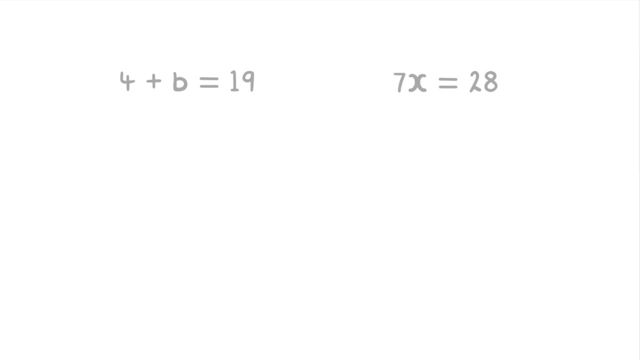 So you can think of it as being a plus 4.. Which means that to get rid of it we just subtract 4 from both sides. So on the left the plus 4 and minus 4 are the same, So you can think of it as being a plus 4..